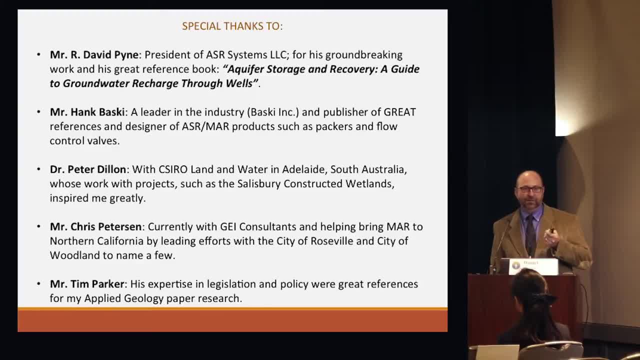 in this region And somebody in the audience, Mr Tim Parker. He wrote Tim Parker. He wrote some papers for previous Bismarck And I found him in the proceedings and asked his permission to use some of his work. He's an expert with as far as regulatory and some of the directions, the new legislation. 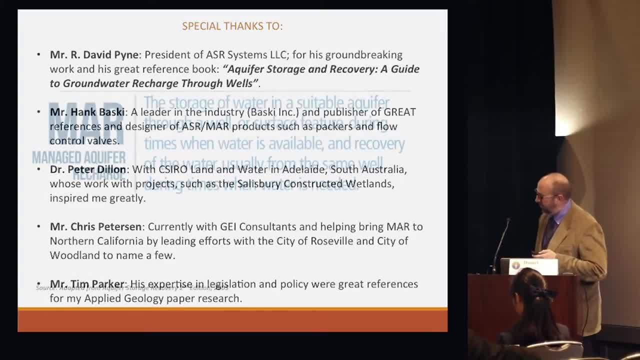 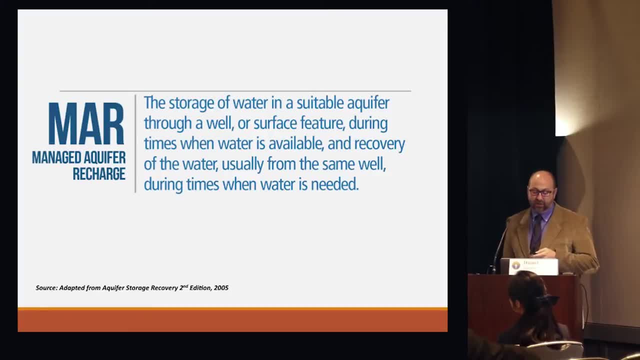 is going And we are trying to streamline the process for managed aquifer recharge projects. So you've seen a couple of definitions already. You look for a suitable aquifer, You try to get water in there. You get water in there via a well or surface feature. 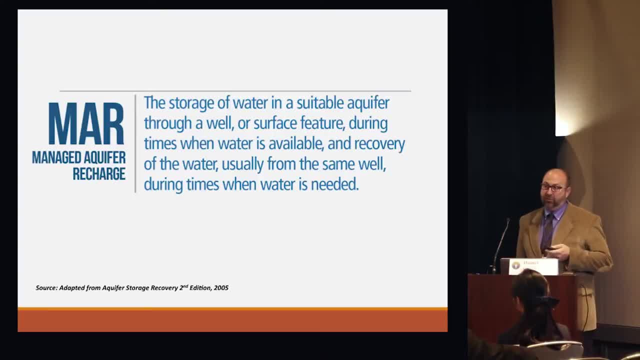 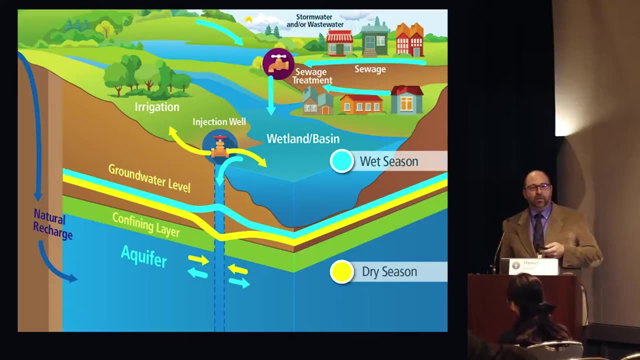 And you try to recover the water when you need it, hopefully in a dry year, And you get the water in during a wet year. That's pretty much it in a nutshell. Here's a kind of conceptual model. I tried to tailor this for agricultural water topics, you know, and so, as you'll see, a lot, 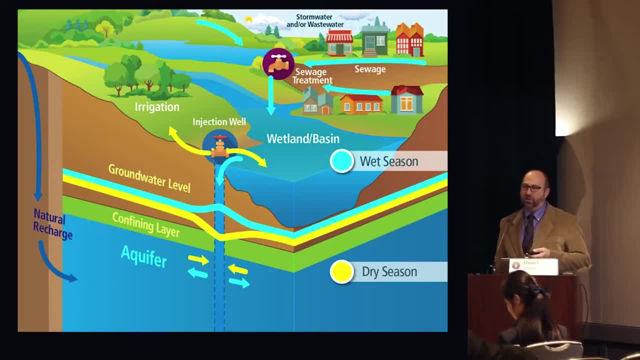 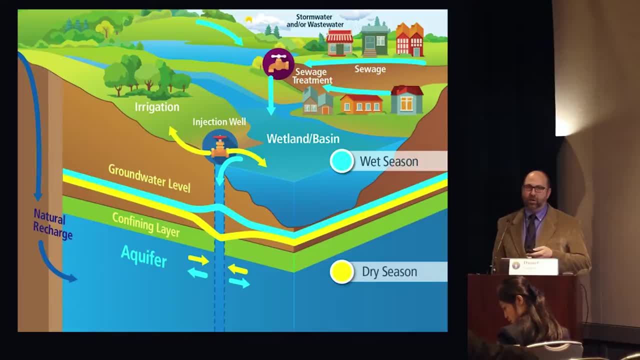 conditions due to too much pumping or, you know, problems with the pumps. so much We've got street water intrusion or we have land subsidence- some of the big issues in the Central Valley. I think we've all seen the picture of the USGS scientist standing next to a telephone. 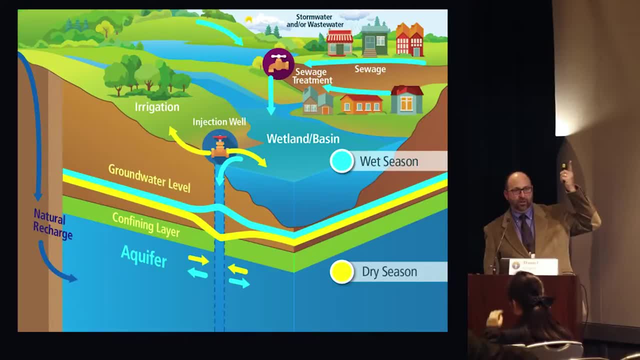 pole And there's a sign. I mean an area where it used to be land surface, and 28 feet below below is where he's standing now. so we have some big problems. um, as, as lester snow says- i think- i think i got his name right- that we have a lot of storage space waiting for groundwater to be. 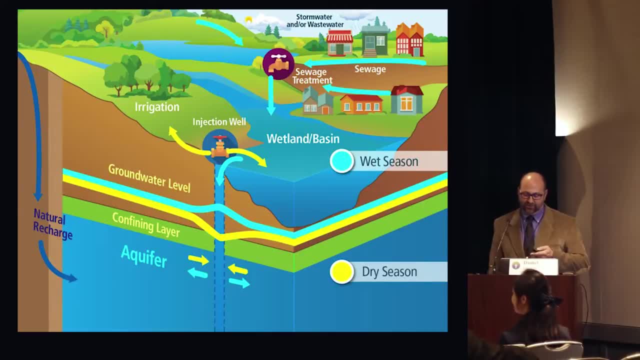 put into it. we've done, we've done a scientist a favor there with some of our practices um wet season and then it comes out in the dry season, as you can see on this, you see some irrigated lands there, wetland basins, treated water, all different types of sources that are. 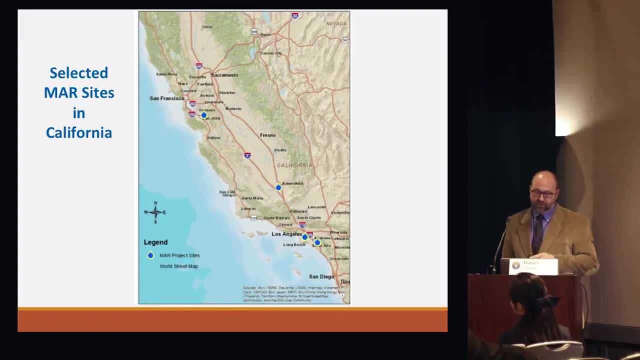 becoming more and more available for recharge. here's some selected sites that i put into my paper. we have orange county water replenishment district. we have that's spot over there by bakersfield- i'm going to talk about the kern water bank- and then we have santa clara valley water district, orange county and santa clara water district. 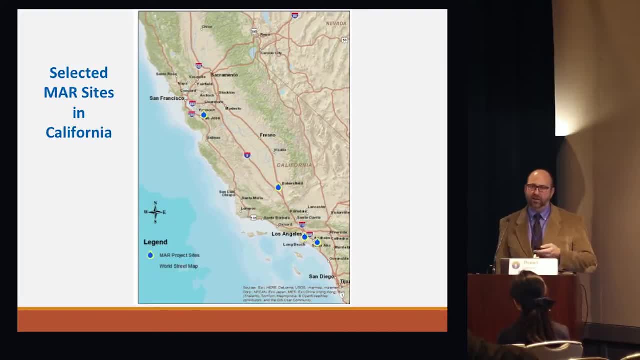 they've been doing this for over 60 years, so there's a lot, a lot of good industry experience there, a lot of expertise, and i think california has a lot of potential to get this into- maybe the more of the agricultural community. the reason i brought this topic is that there's so many. where are the wells at? where are the? 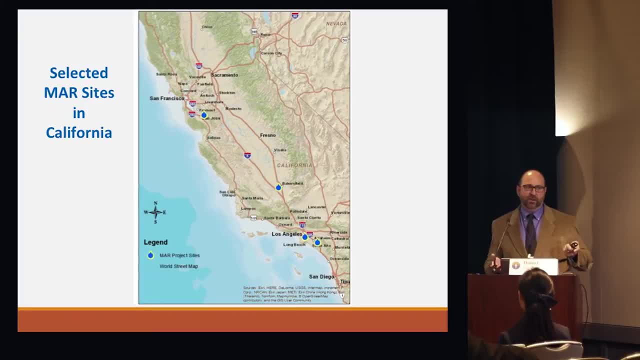 straws to get water into the ground. you know it's usually on these agricultural irrigated lands. they have all the wells, they already have a lot of the infrastructure. they have a lot of the power supplies there, a lot of the roads, so maybe they're going to be a player in the future. 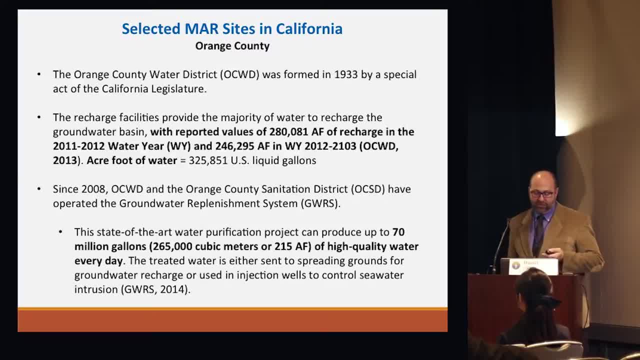 just as an example of a of an area- orange county water district- formed in 1933 by a special act of california legislature. legislature probably would not happen as quickly as it happened then. in today's regulatory and legal environment i think that needs to change, but it sprang out of necessity. overdraft seawater. 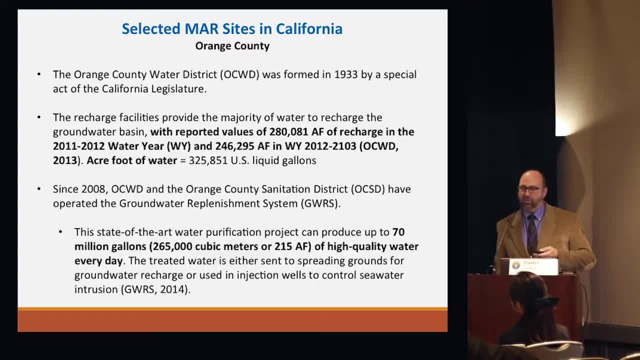 intrusion, lots of people fighting over water, falling water levels. so now they have a system in place that gets about 280 300 000 feet of recharge per year and a lot of that comes out. they have a base pumping percentage that they set, so they have freeboard. they work within a range. 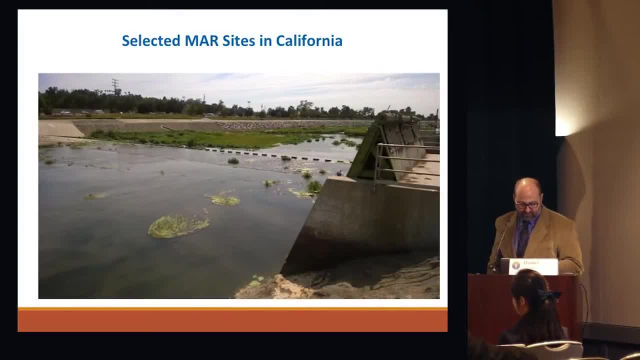 you know. so they don't want to get it too full and they don't want to get it too empty. thank you, we went on a tour there. this is like just one of their spreading grounds canals, you know, with the weir system, and this is just one of their many channels and canals that they get the water into. 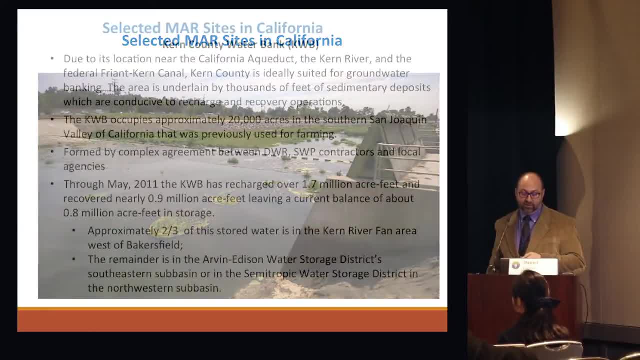 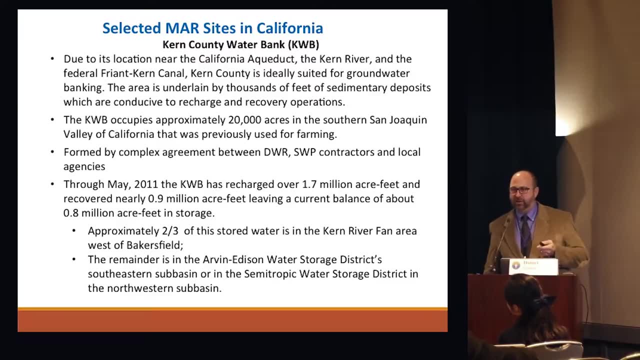 they do this year in and year out. it's amazing what they do there. the kern county water bank- it's up there in oil and gas country and farming country north of bakersfield. it's also hydrogeologically suited for recharge because there's thousands and thousands of feet of 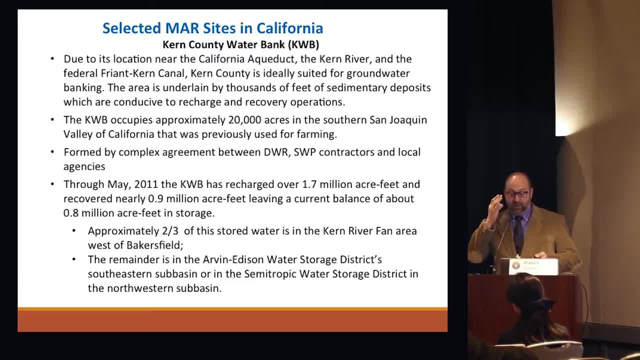 land that are conducive to recharge in this area, and it's just really blessed by its location to the aqueduct, the kern river, the frank current canal and all these uh appurtenances that can get water to it, and um, so they got together. there's a complex agreement to kind of fallow. 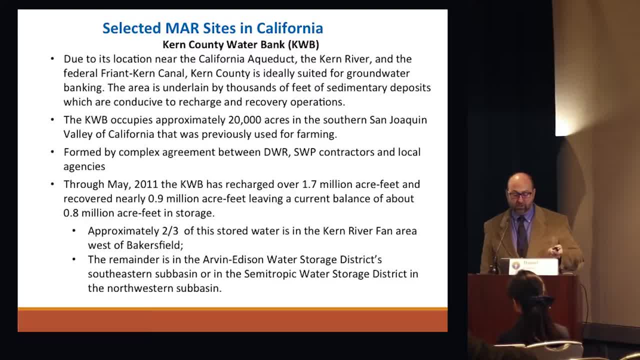 a lot of this land or take it, take it out of agricultural hands, with the promise of using as a water source the department of water resources, the state water project contractors got together, they hammered out something i think was called the monterey agreement and they formed this complex water bank. 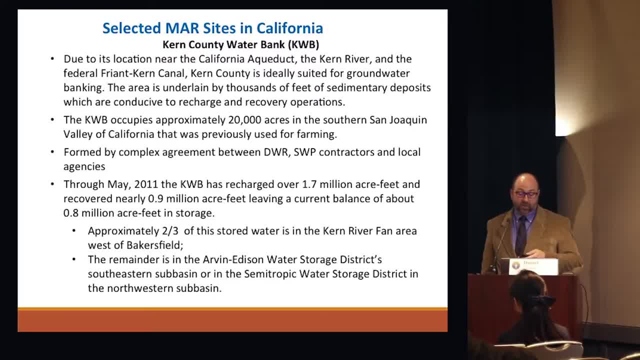 and they've gotten about. they said they've recovered about 9.9 million acre feet, that's, as of 2011, probably a lot more now. so what they do is a very complex system of water wheeling, water trading negotiations to get the water in the ground and to get it into the aqueduct during dry years. 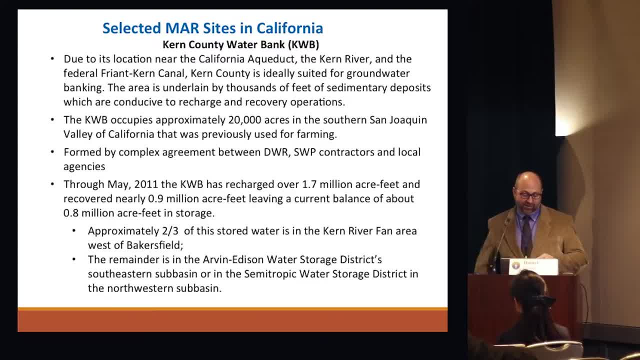 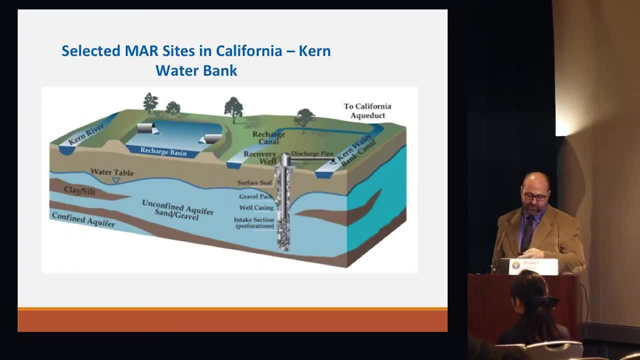 they're just it's very complex. it's it's like a water bank. you know it's like a big time, you know moving money around, they're moving water around. it's pretty fascinating. and this is kind of a conceptual picture of what they do there. you can see the kern canal, the kern. 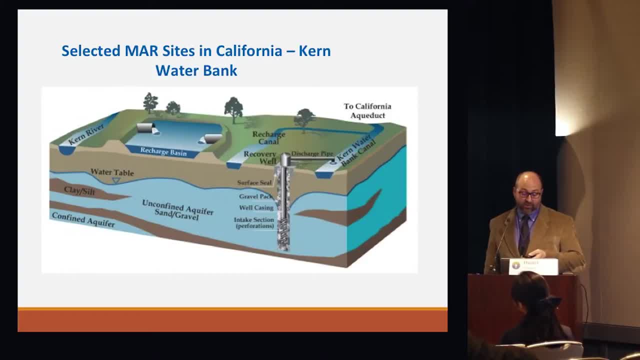 River, the aqueduct, and that's kind of what they do. they get it in the ground and then they have recovery wells, and they have hundreds of recovery wells that get the water into canals and the aqueduct for for buyers downstream, and what this was was 20,000 acres of irrigated land, farmland. 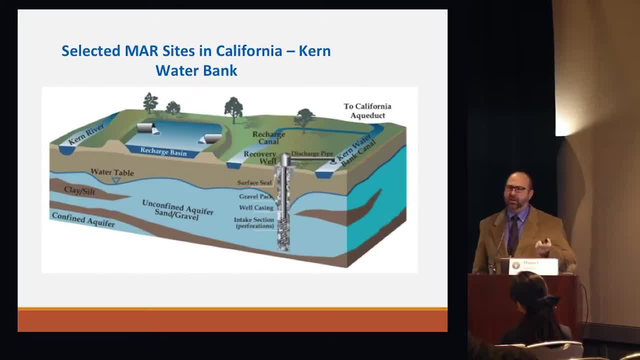 that has now been used for a water bank. so kind of goes into the potential. you know, the potential for for California to get out of our large critical overdraft situation I think exists with a union between private entities, public entities. when I say private entities too, I'm 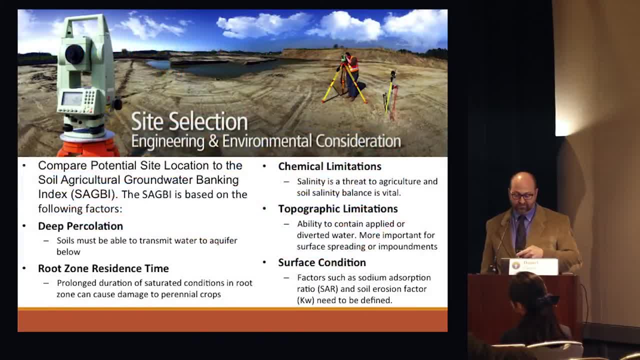 talking about private pumpers, private landowners. now to getting some of the more of the planning aspects of this site selection, the UC Davis AG extension, along with some consultants they hired and some, maybe the, I believe some of the Water Education Foundation and and maybe Water in the West, some kind of 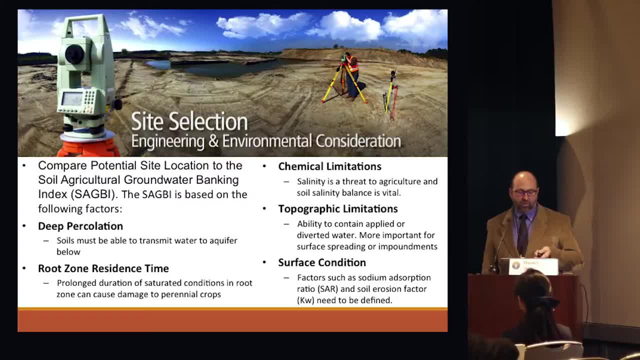 non-profits got together and came up with a Soil Agricultural Groundwater Banking Index. it's- it's online now. it's. it's a. it's a web application that you could use as your first point of contact or research and they look for suitable recharge, surface, recharge areas and you can almost use it. 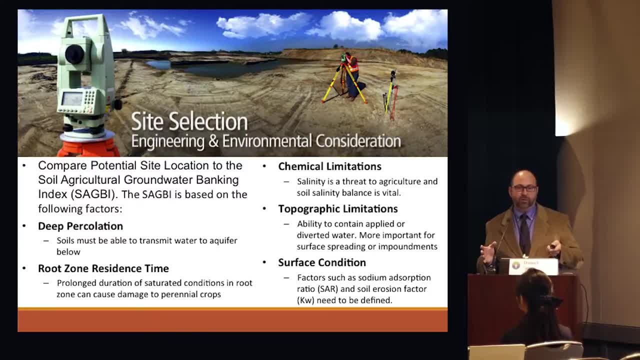 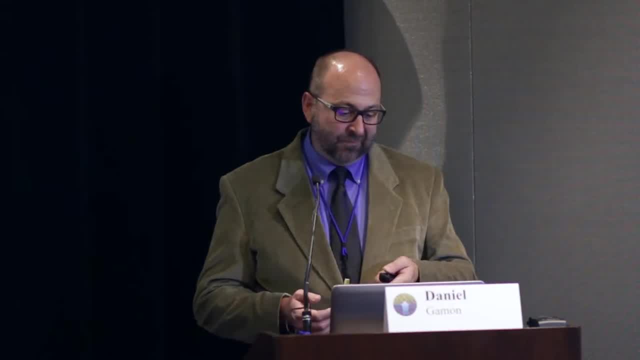 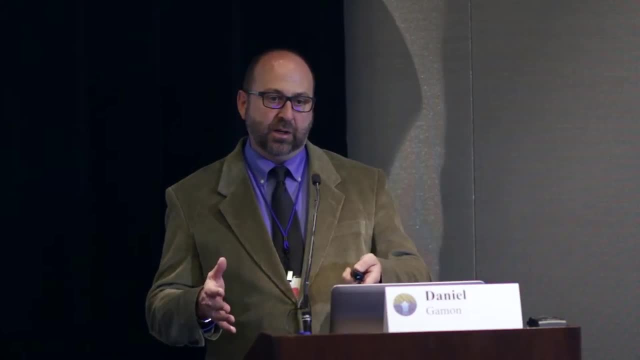 too, for groundwater recharge research too. if you want to find some groundwater recharge sites- and they're looking- the following factors they look at is deep percolation. you know. obviously if you want to get watered down into the aquifer it has to have that good vertical connection, the root zone. residence time. you've been hearing that a lot in the news right now. what? what plants or perennial crops can take long-term surface water, flooding or diversions, you know? I think they're saying grapes are pretty good, almond trees are pretty good, maybe walnut trees or something else. not so good, they don't. like having their roots soak that long, so that's something to take into consideration. Central Valley salts are always a problem. you have to worry about your water chemistry, your water mix, mixing models, topographical limitations, if you're going to use surface water and then pound it or 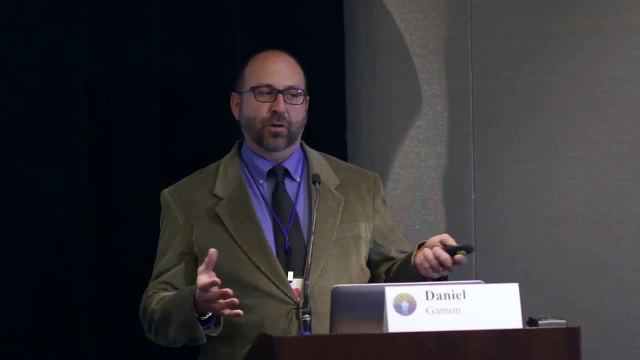 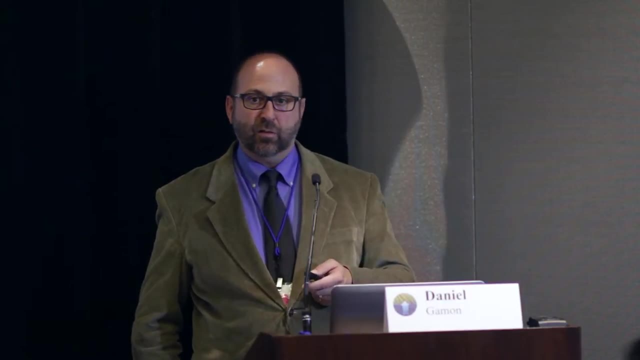 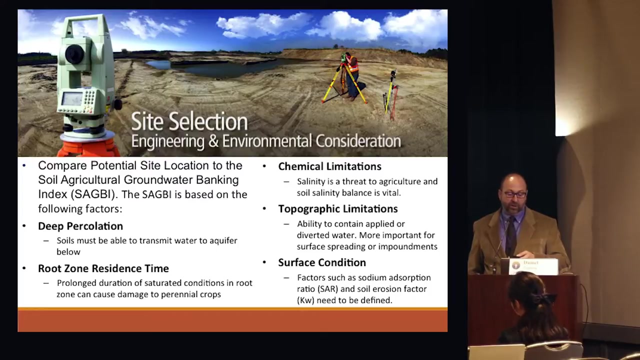 divert it, make sure it stays where you want it. to surface conditions. this kind of gets into the soil chemistry and the mixing models. you want to know what your sodium absorption ratios are, the erosion factors you know, and just how is this going to hold up to long-term flooding, drying. 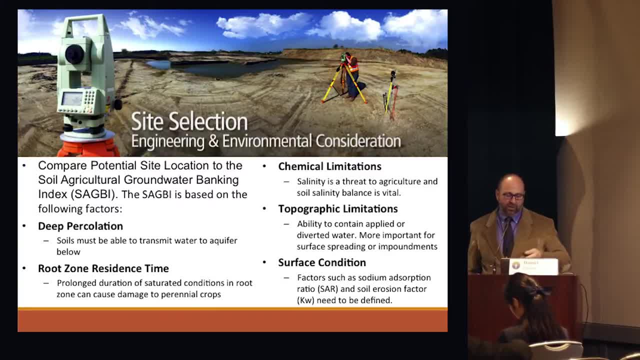 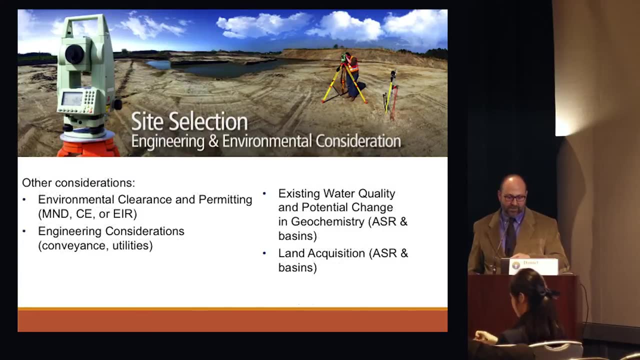 cycles: flooding, cleaning out and then flooding again. so Orange County Water District, Santa Clara Valley Water District, are really good models there. they have a lot, of, a lot of good online information or documentation, more site selection stuff. you know, obviously, if you're going to get into the planning. 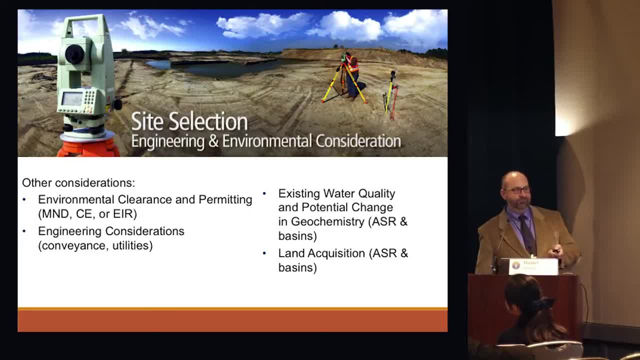 you know, plan to succeed, don't plan to fail or fail to plan something. you know you've heard, heard those, so just make sure if you're going to use- like I work with some AG clients and right now, some projects, it just brings up all these regulatory red flags, unfortunately private pumpers or private 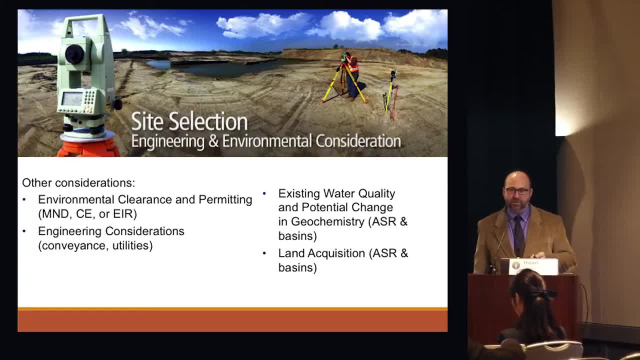 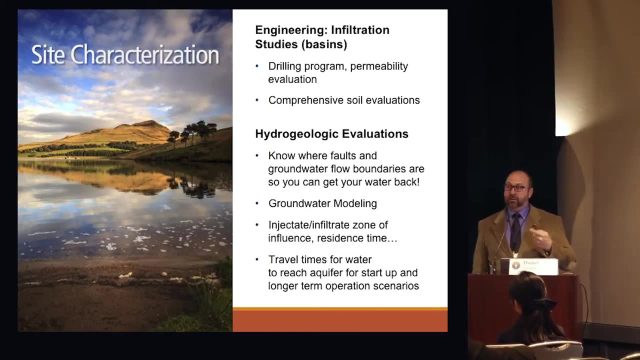 landowners seem to run afoul more of the regulations than public agencies, and it's too bad because a lot of these people do want to do sustainable type of projects. obviously you want to get out there, start doing your field studies. a big one is: know where your faults are, know where the groundwater is going to flow to. 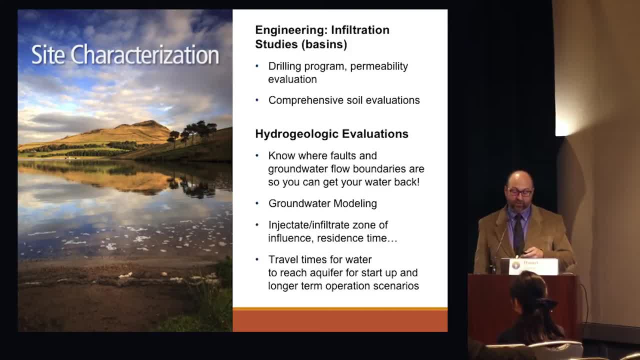 there's a couple pretty pretty- I could do a whole slide on a couple of case scenarios where there is success and there's abject failure, because they didn't map faults and groundwater went where it wasn't supposed to go and the recovery wells were, you know, sucking air. 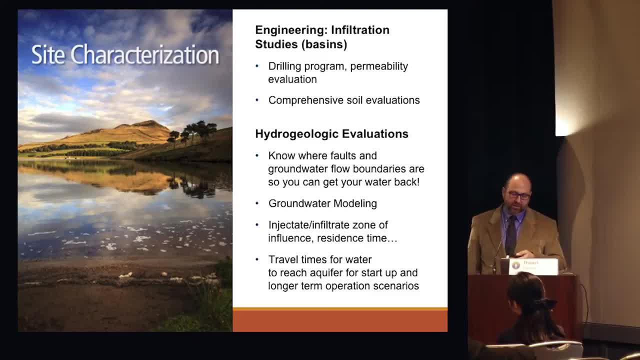 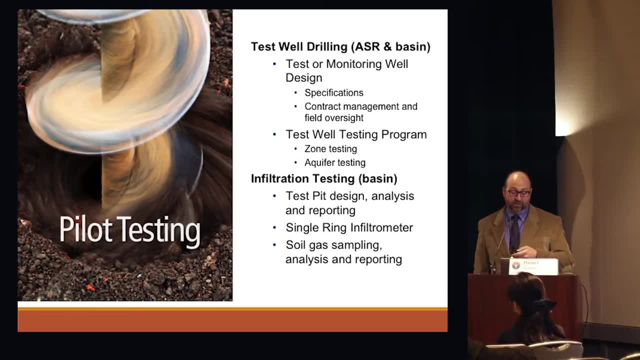 so to say you don't want that to happen? test well drilling. this is for your ASR and basin studies. you want to? I could do a whole session on the technical aspects of ASR well design and I won't bore you with that, but there's a lot to it. I'm 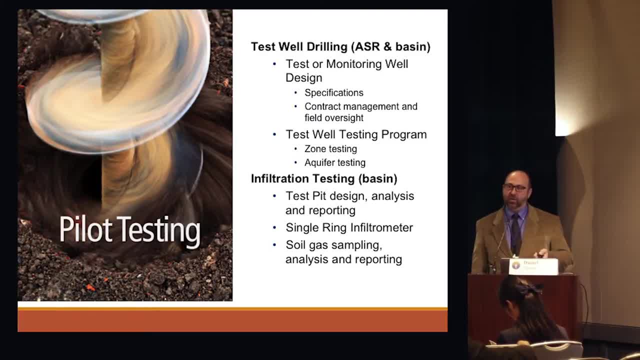 really skimming over a lot of this. but ASR wells- recovery wells are different than just pure pumping well design and that's what I'm going to talk about in a little bit. but I'm really skimming over a lot of this. but ASR wells- recovery wells- are different than just pure pumping wells. recovery wells are different than just pure pumping. 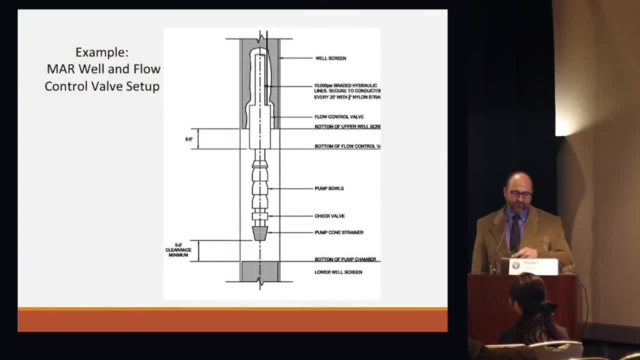 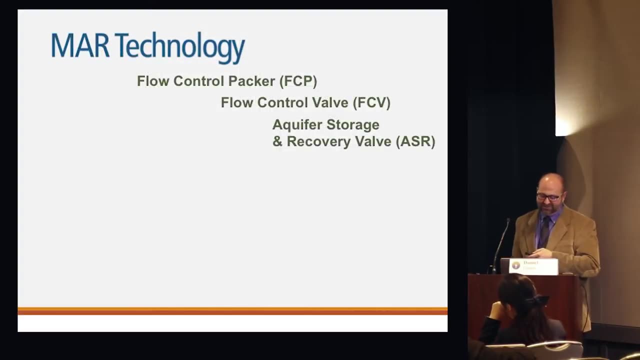 extraction wells. here's an example of a. I'm gonna get into some of the extraction wells. here's an example of a. I'm gonna get into some of the technology. but here's a managed off a recharge well with flow control valves and that gets into more technology and 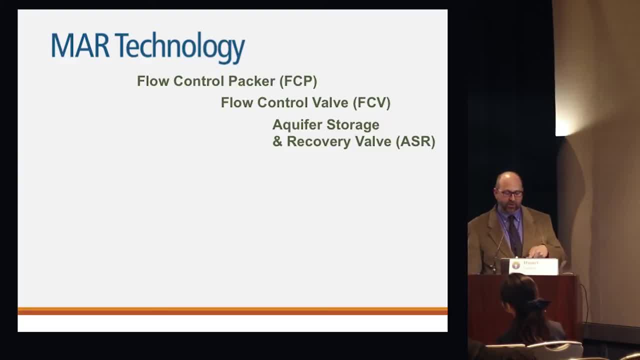 basically to control your downhole flow. you're going to either use Packers flow control valves or more advanced aquifer storage and recovery valves. and Oxygen turbulence- all that are the enemies. You want to have that smooth flow. You want to keep the oxygen out. 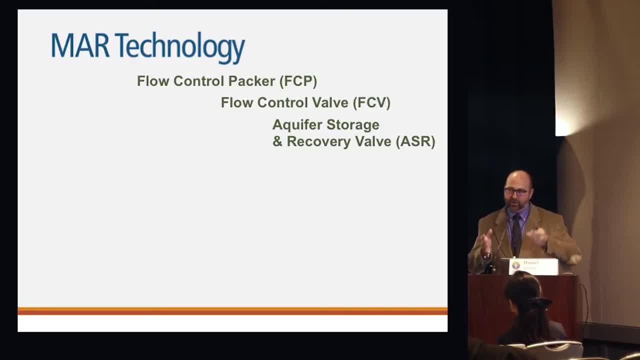 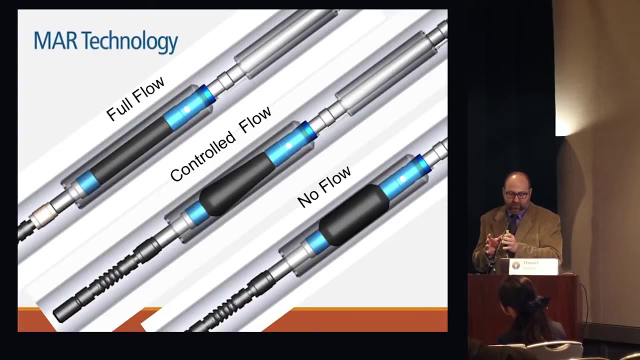 You want it to be. you don't want to create a vacuum, You want to get that water in the ground and you don't want it to be disturbed. so you have geochemical changes taking place. So here's some packers: full flow. the packers closed. 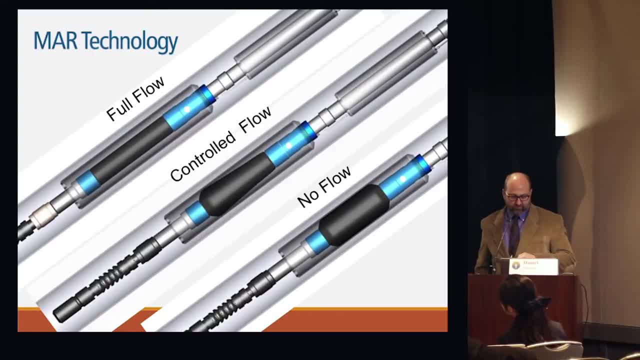 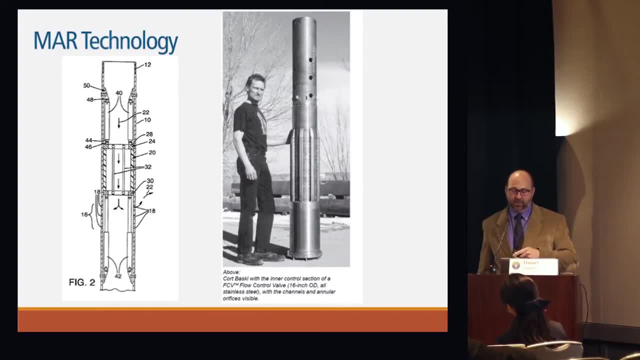 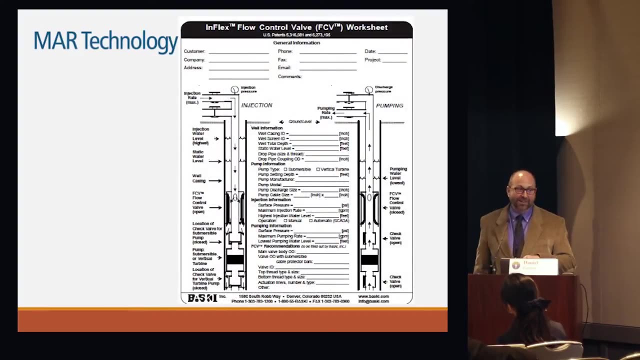 No flow, the packer blows up. Talking about the Baskies, here's a big flow control valve you can put in line in a usually a turbine pump system. Here's a worksheet. don't worry, there won't be a test. 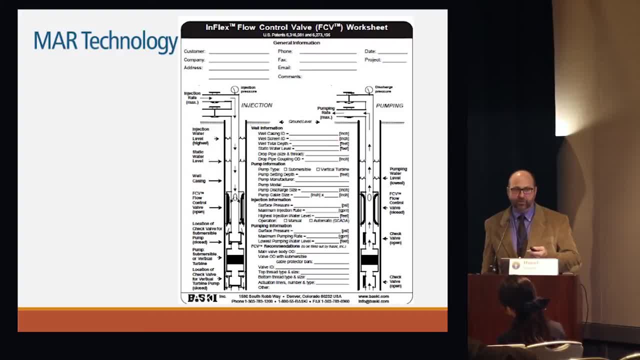 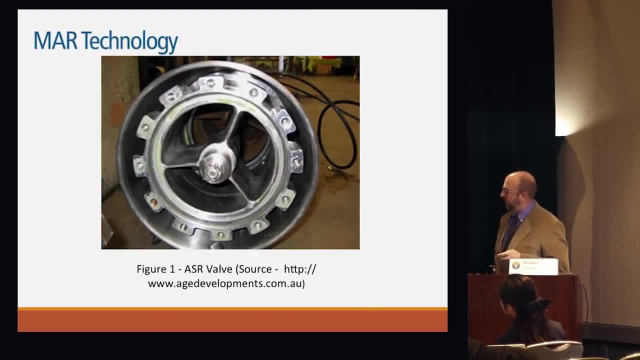 That's just to kind of show you some of the planning references or tools available out there that go into this for a successful program. Got to give my a shout out to the Aussies once again. Here's AG Development. They have an ASR valve. 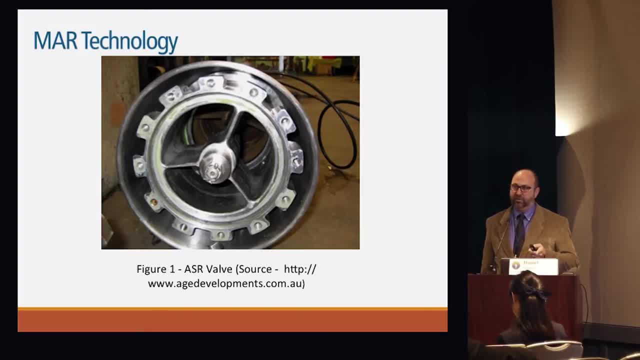 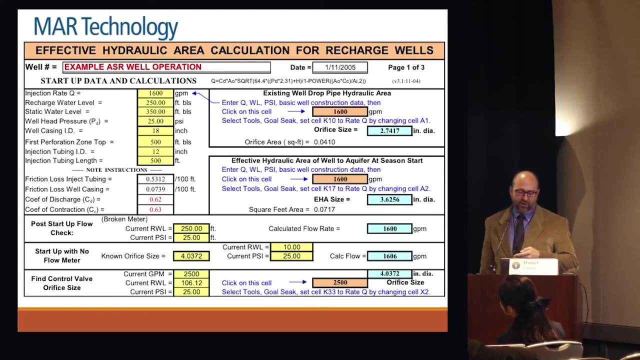 They're out of Western Australia and this is pretty much state of the art for flow control: down hole and to it rotates and allows the water to be extracted. Here's kind of an example for startup calculations. You know this is the type of worksheet. 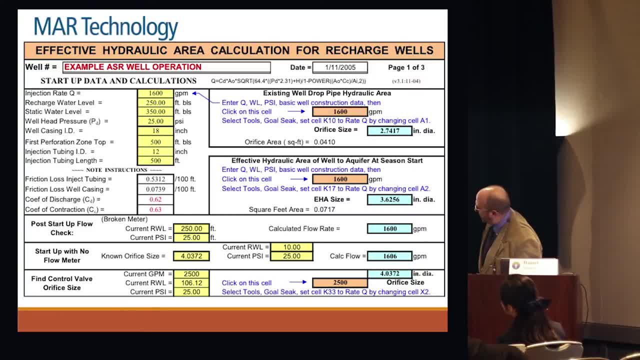 That's developed. it's name didn't get in there, but I think this is from Tony Scott. He runs the Los Angeles ASR well field, one of the biggest ones in the United States. He was trained under David Pine- excellent source of knowledge and experience. 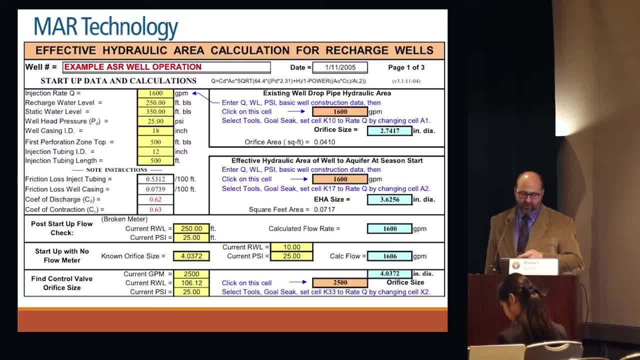 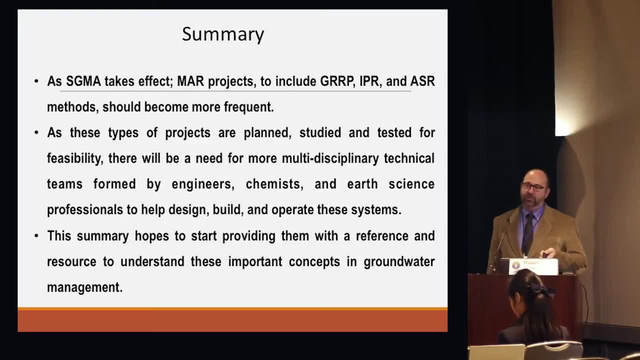 So what I geared this to. in summary, as a sustainable groundwater management act takes effect, I believe more projects will be to include groundwater replenishment projects, indirect potable recharge, aquifer storage and recovery. I think these methods will become more frequent. 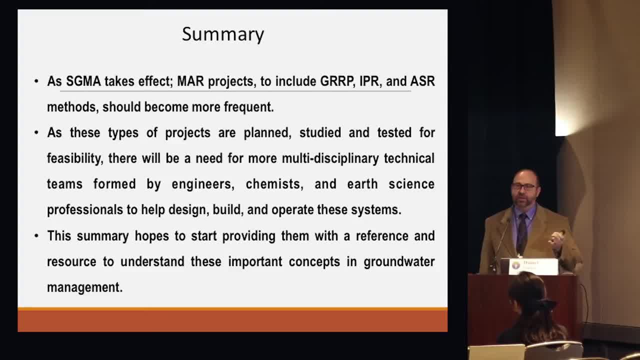 I think these type of projects we're going to need more professionals. It's multi-discipline, you know: engineers, chemists, earth scientists, process engineers, mechanical engineers, Hydrogeologists, groundwater modelers, geochemical modeling. this all goes into a successful 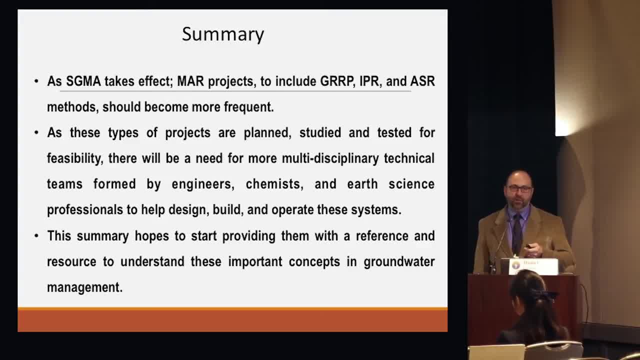 program. So get a good team right off the bat, do a really good feasibility program. a lot of pilot testing, bench testing keys to success, And so I hope this provides you a reference and a resource to understand these concepts in groundwater management. 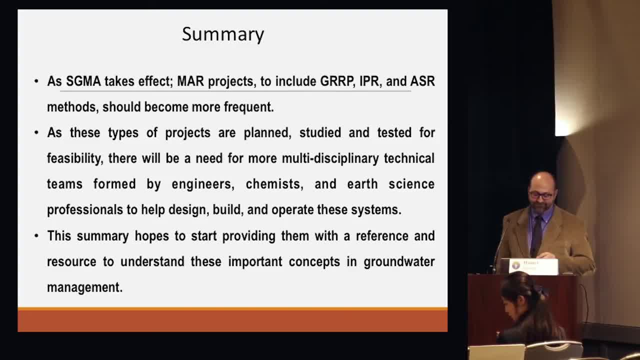 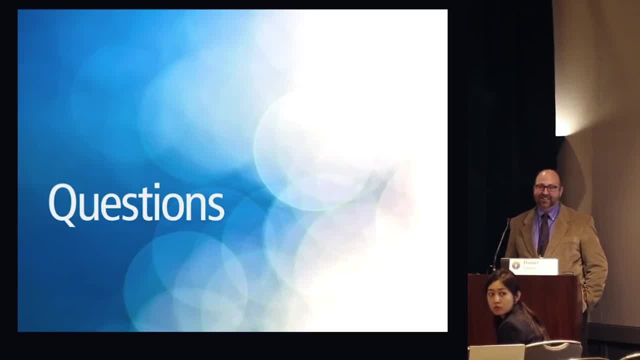 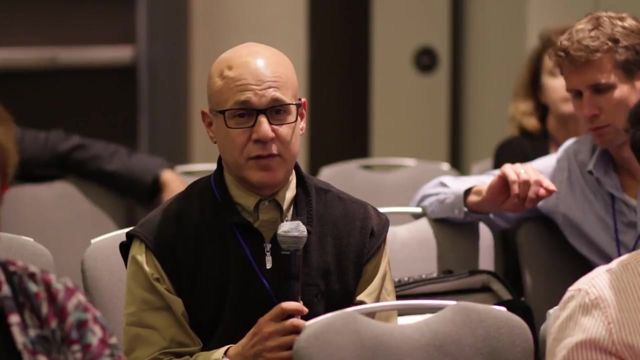 And thank you. Are there any questions? Hmm, There's one A little more popularity. just one comment on something you said which I think is important about: you should know where your water's going from too and plan for that. I think that basically, is very true for MAR projects. 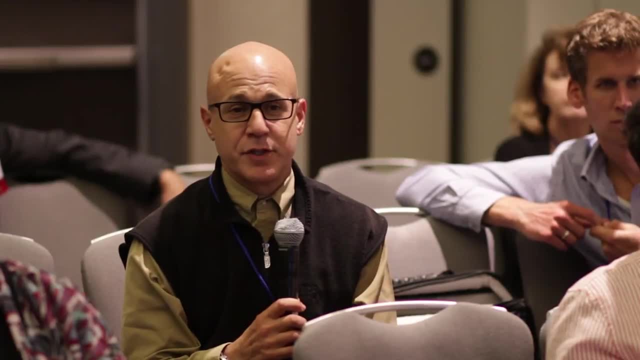 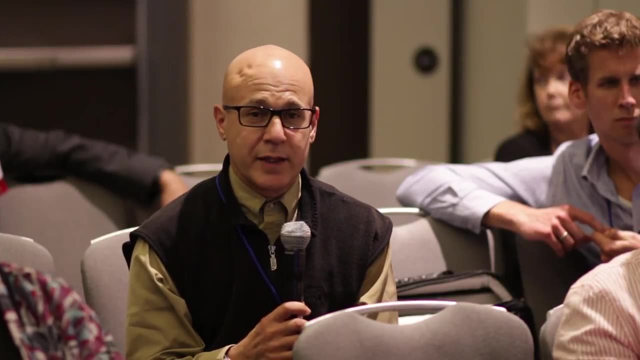 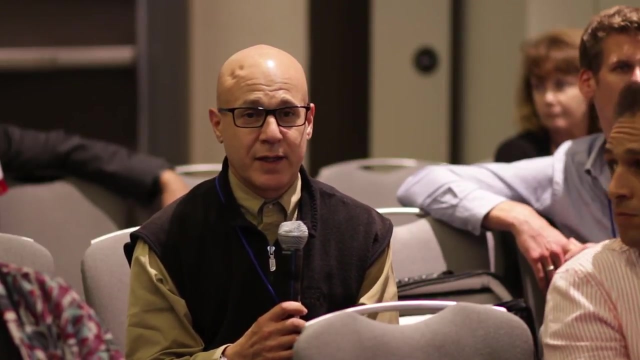 But incredibly true for all sorts of other hydrogeologic projects which I think people really miss the importance of, whether it be for a production. well, modeling, that you really need to have a good conceptual model And I think that not enough time is spent on that and that you really with a good conceptual model, that's an incredible building block for the rest of the project. 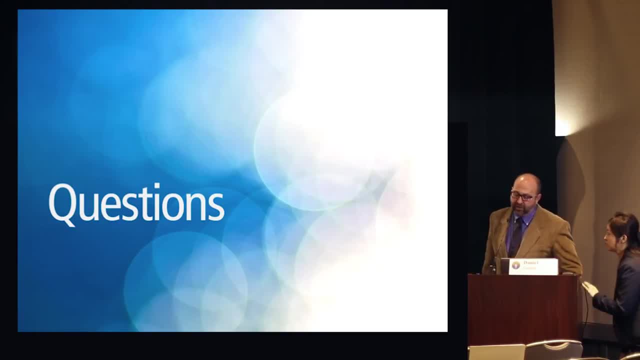 So I compliment you on pointing that out. Thank you, I totally agree, And one of the resources we have for conceptual models are those wells that are drilled out there by the private pumpers who have the majority of the wells, and if you could get other well logs. 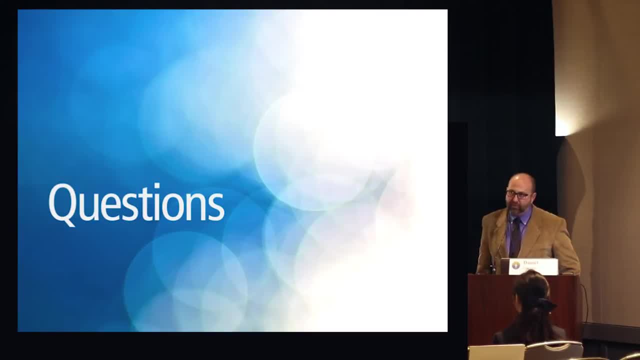 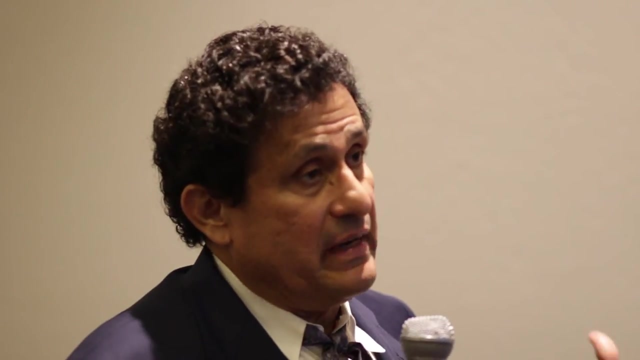 But that's what I think. SGMA in general is going to be built on: good hydrogeologic conceptual models. Any other questions You go? Yes, my experience with recharge. I'm familiar with the Orange County one and the one in Kern, Alluvial Fendt. 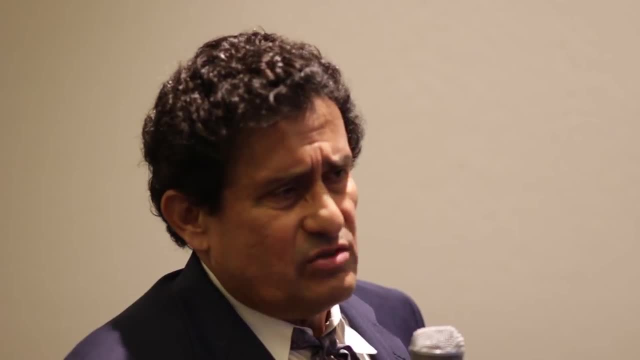 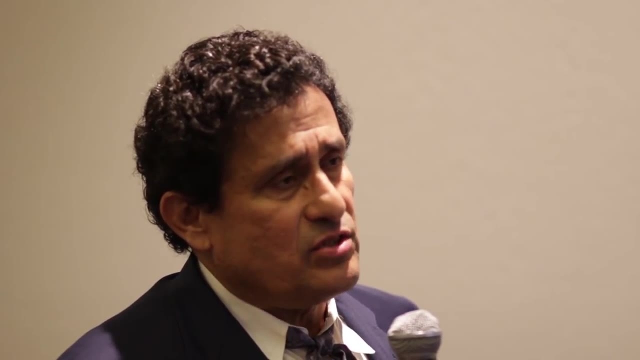 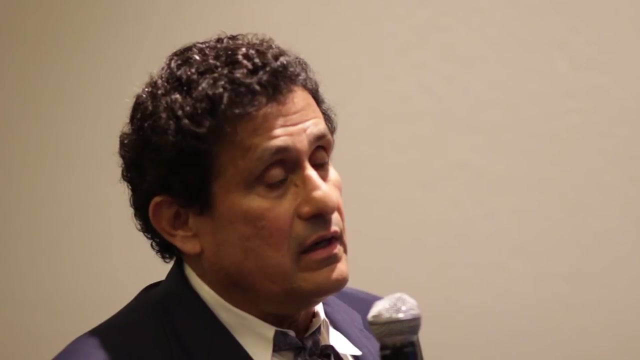 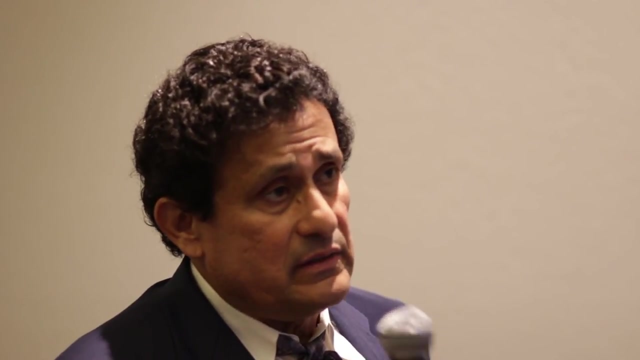 You mentioned a well field somewhere in the Los Angeles area- I understood Las Vegas, Okay. Have you seen any successful large-scale injection using wells? Because it's not an easy operation to recharge a lot of water with wells hydrogeologically. So have you seen any successful operations in that respect? Mostly, like you say, it's small scale and then the large-scale Las Vegas, I believe they get in 500,000 to a million acre feet, maybe less than 500,000 acre feet, and it does. It's a large amount of infrastructure and a large amount of operations.